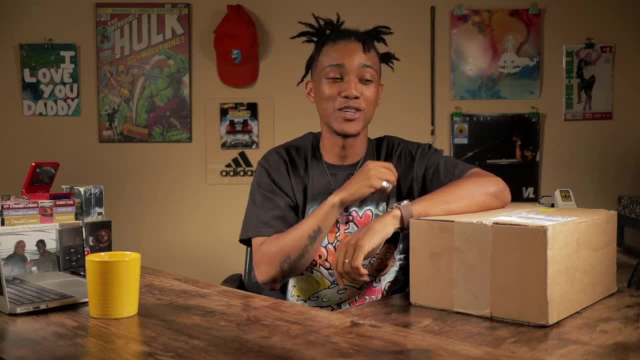 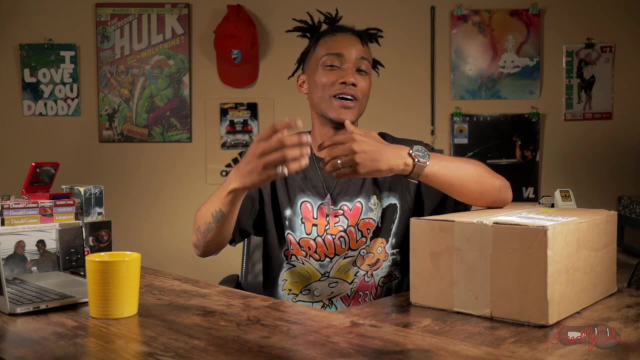 for you How y'all doing today. Hope you like my last video. That took me a lot of effort, a lot of time. It was very different. It took a lot of heart for me to release those songs and release that different. 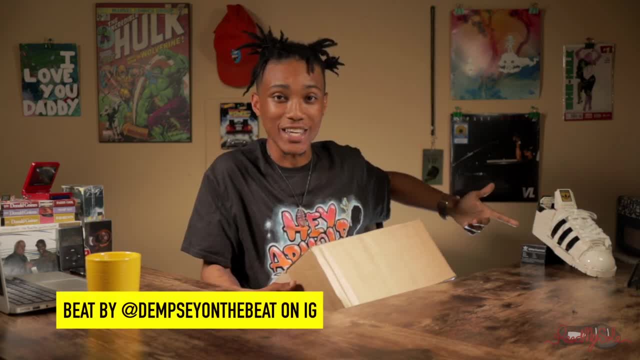 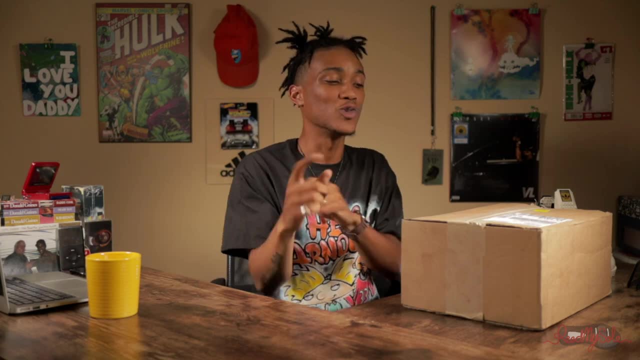 But I hope y'all like it. I have the superstar back here. As y'all can see, it's part of my setup. I hope y'all like that video. But today we have a shoe- a real shoe- review for you. This is a story. Before I get into it, let me just explain the story I ordered. 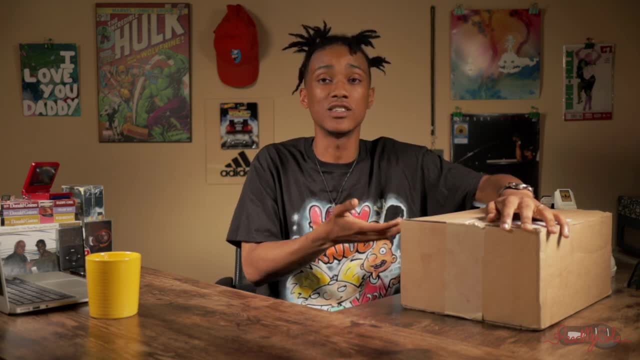 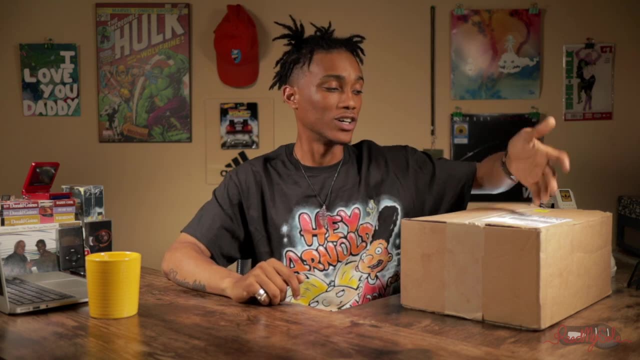 this from GOAT. This is. you see the title. of course this is the Yeezy 450 Dark Slate. I, like everybody else on release day, I got up, tried to get it on the Adidas Confirm app, entered the raffle. big fat L. 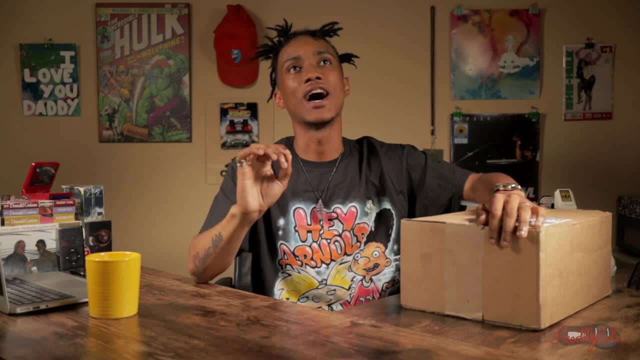 Then I went on Yeezy Supply. I don't even know why I even try on Yeezy Supply anymore. I'ma be honest with you. I don't even understand why I even look at it. It just doesn't happen. 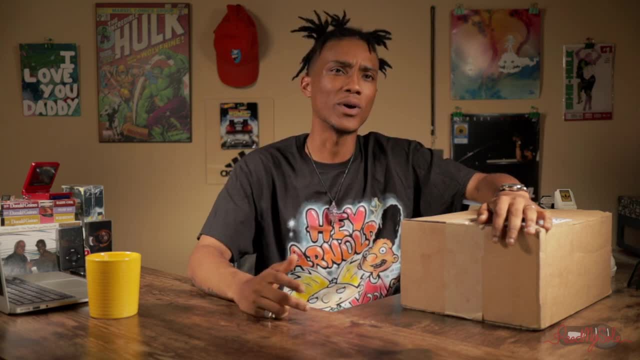 I think I got the Beluga 2.0s on there way back in the day when Yeezys were sitting. I was able to get the 350 Beluga 2.0s on there and I'ma be honest with you, that's like the. 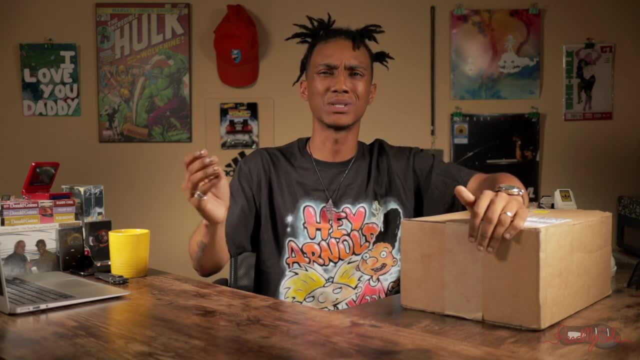 last thing I ever got on there. I got in on maybe the Quantum basketballs, but they kicked me out, denied my card. Yeezy Supply is just a no-go. So, yeah, I took a big L and I really wanted this shoe. 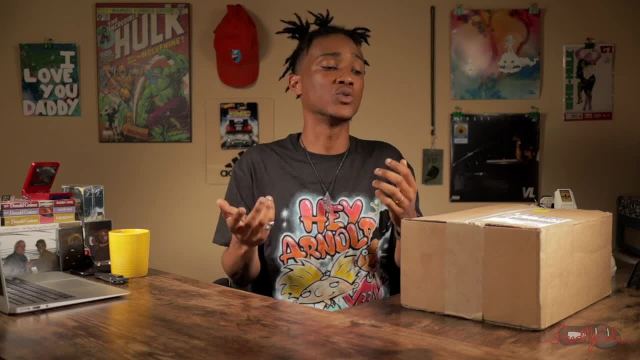 I wanted the cream version, the white version, whatever the first version was of it, and I wasn't able to obtain it, So I ordered it off of GOAT. GOAT had a good price. I thought they were going to be like. 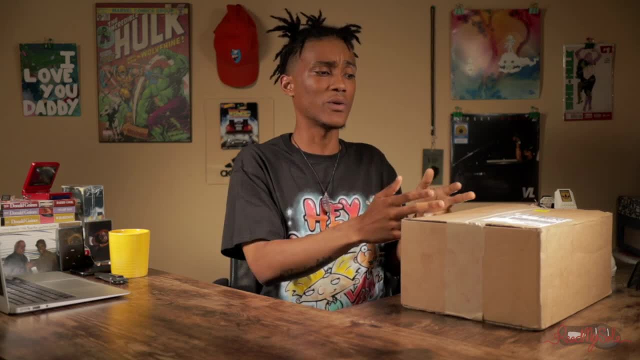 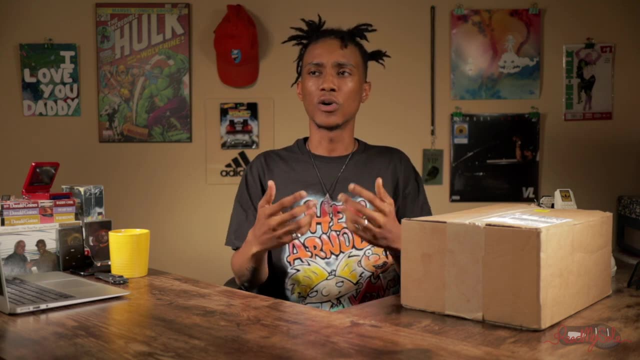 $800 resell- I mean $1,000, and they were actually didn't resell that much. So when I saw the price, which was like 300, I had like a 5% off coupon through my CashApp card. 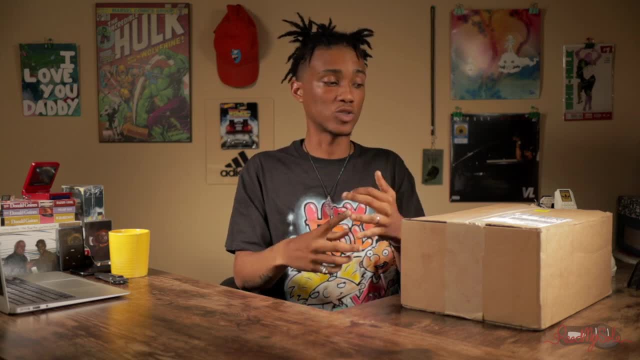 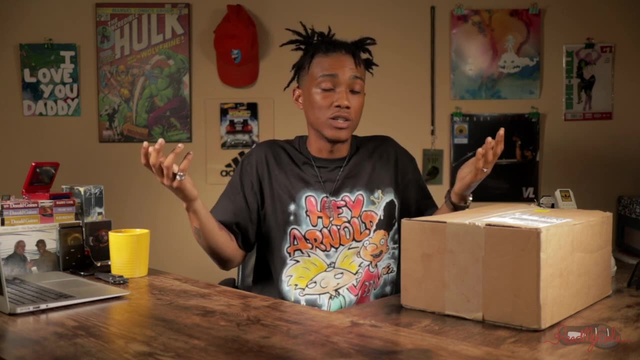 I also had like another. I had a bunch of percentage off for Flight Club and GOAT, So I ordered off GOAT. GOAT took like maybe two or three days and then canceled my order. I don't know why. It was my first time ordering off of GOAT, It is what it is. I had a 5% off. 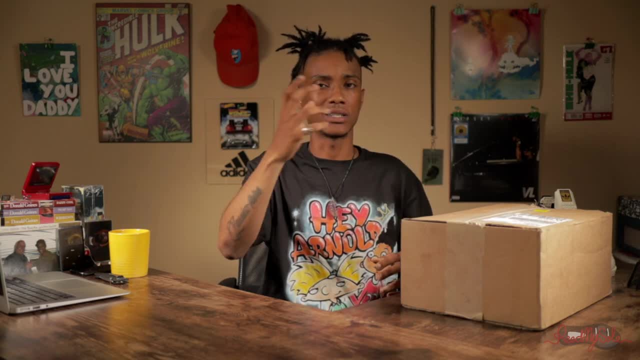 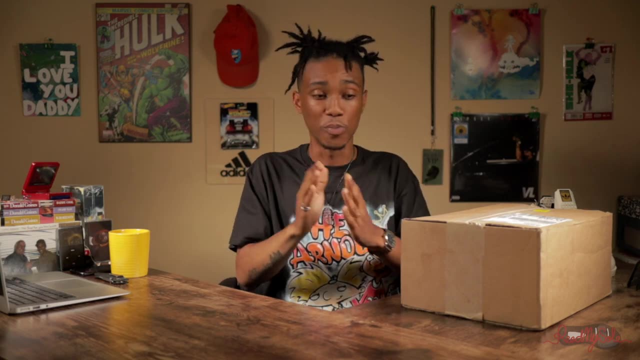 boost for Flight Club and I actually ended up paying a dollar less. I know that's not a lot, but for me paying resale is a no-go. Going to Flight Club is a no-go, But without further ado. I don't want to talk too much. That's the story behind this. I've been waiting. 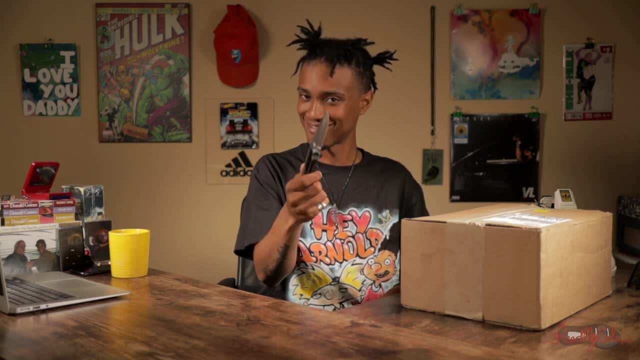 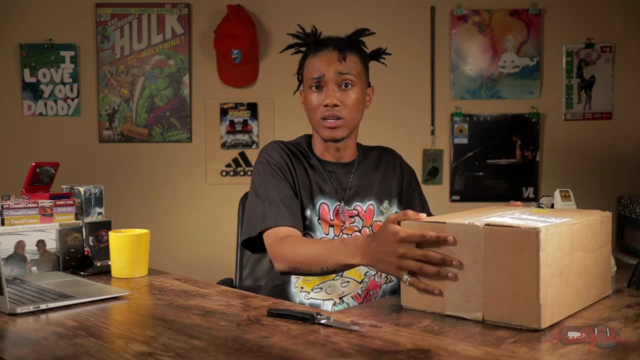 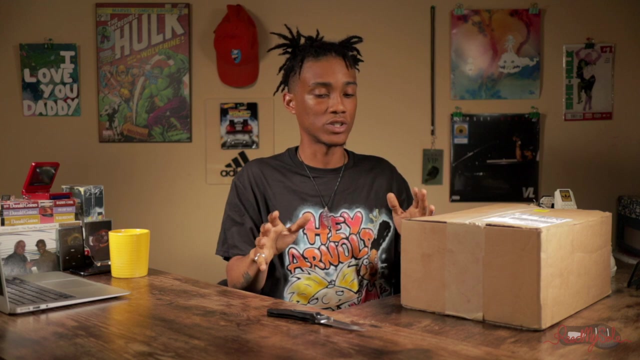 for this. This came from. I have my knife came from London. This came from England. It shipped FedEx England. I ordered this last week and it was here within the week. I ordered it on a holiday weekend. So I ordered it on holiday weekend, which is a no-go, but it was still here within. 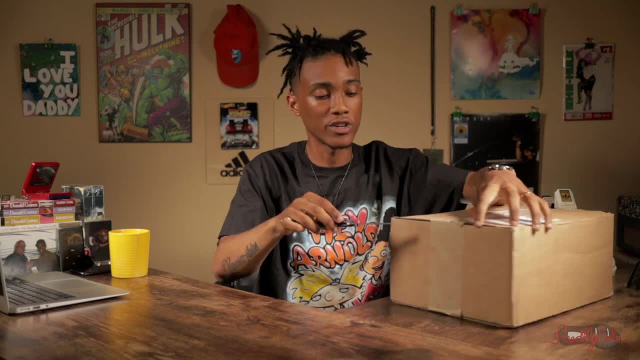 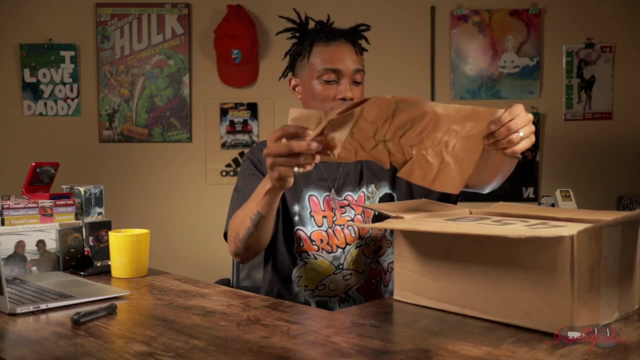 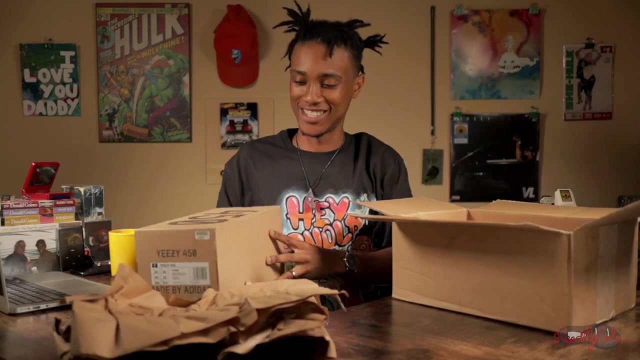 that week, So it came really quickly, Without further ado, let's get off into this. Shout out to Flight Club: of course They put some extra paper in there. They put some extra paper in there Because this is a small box. Whoa, this is definitely a small box. 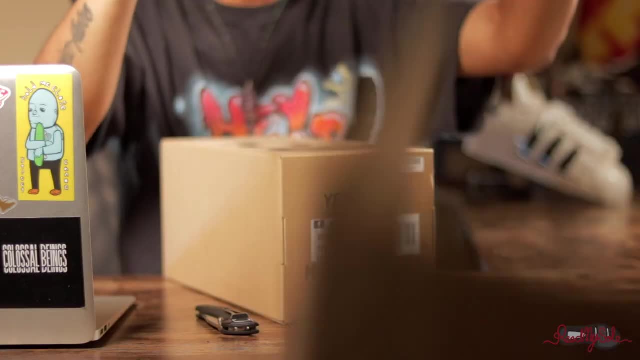 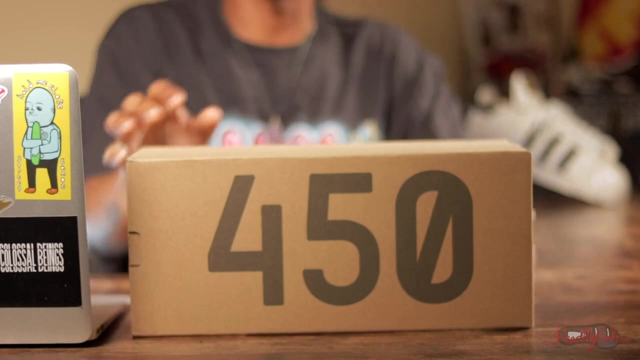 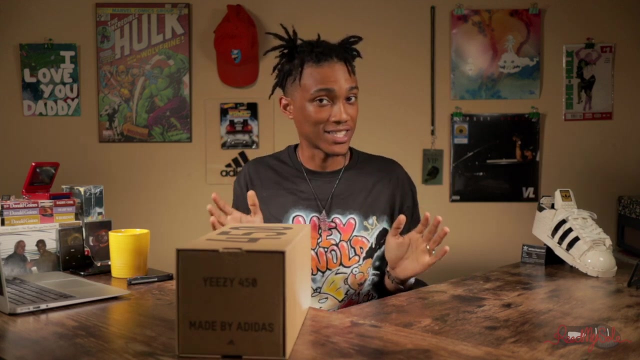 the box. let me get this a lot of hay. this is the Yeezy 450 box. as you can see there, it's a small box. I actually listened to the reviews this time and I went up to a 10 and a half. you know that's. 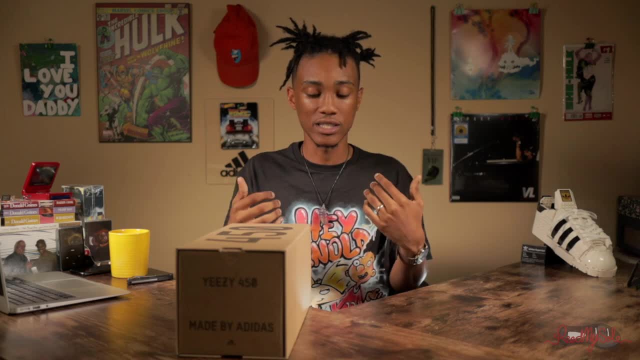 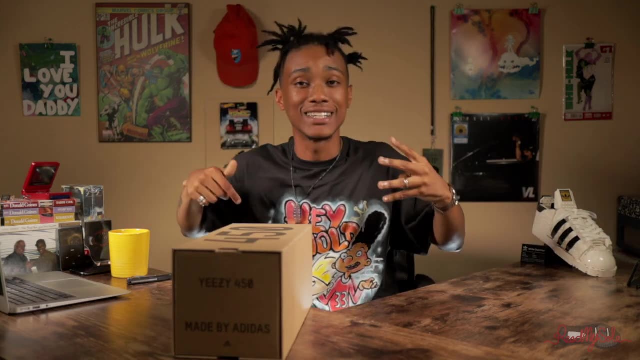 not my size. y'all know I always say that's my size, that's my size, that's not my size. I actually listened to the reviews. this time, hold on, let me take these. let me take my uh, all-time favorite Jordan off. let me take those off because I'm ready to try these things. I don't have a 10 and 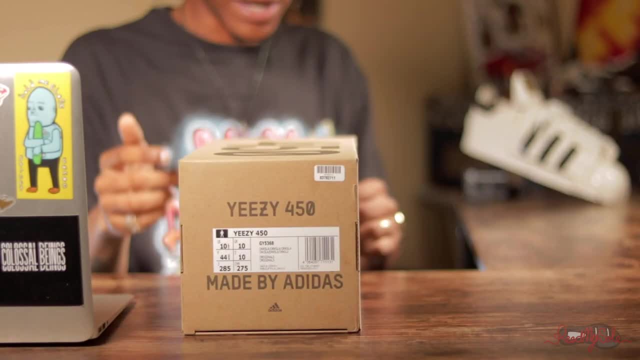 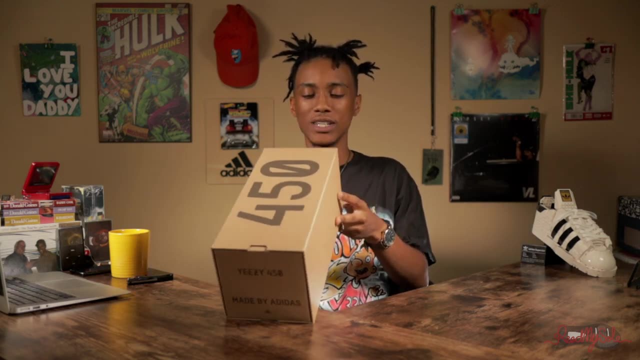 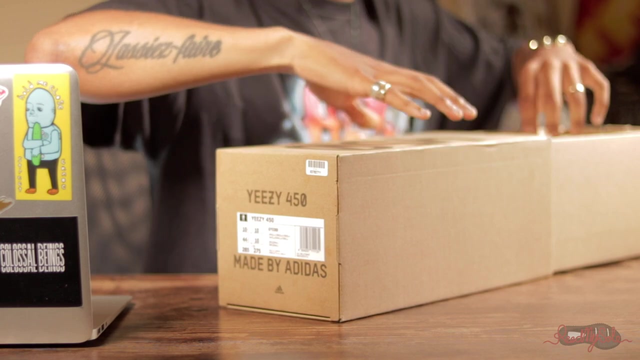 a half right there. I don't know if you can see that it's the Yeezy 450 made by Adidas. yo, I'm excited about this. I'm excited about this. these were made in Germany. I hope these are legit. man, I ordered it. this is my first time. oh yeah, this is nice. this is nice. oh so we have, we have. 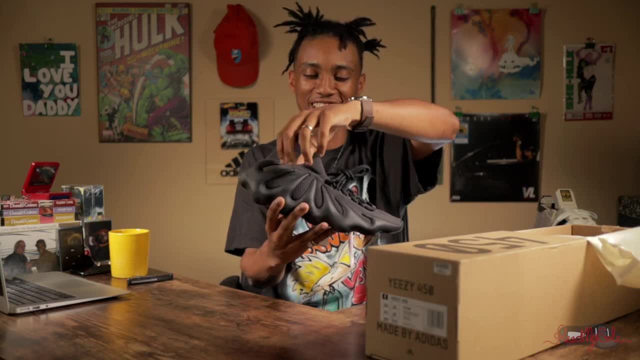 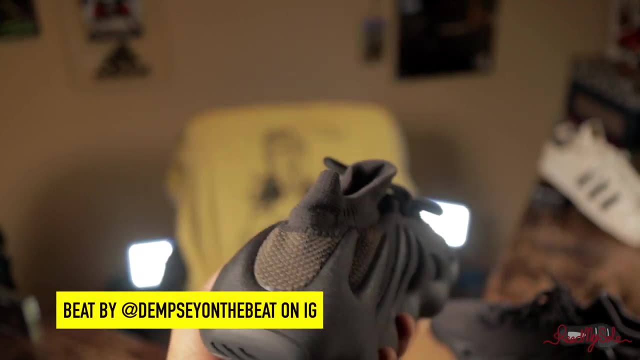 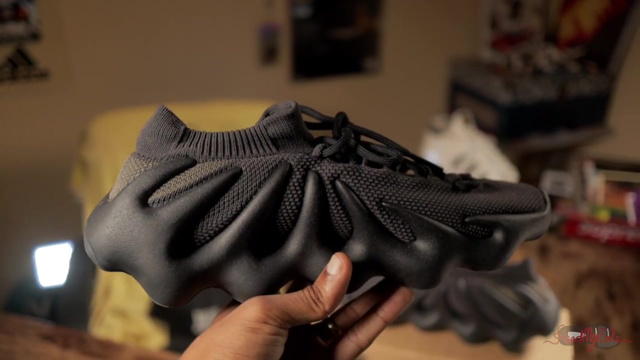 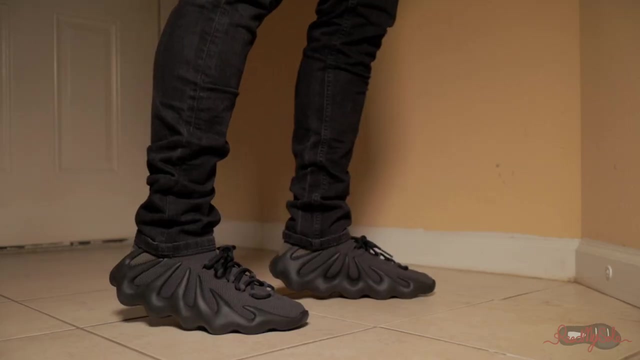 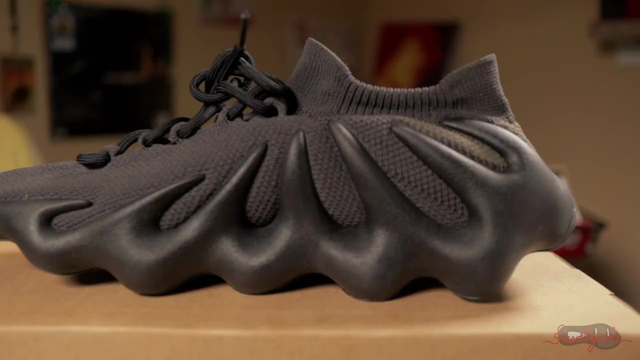 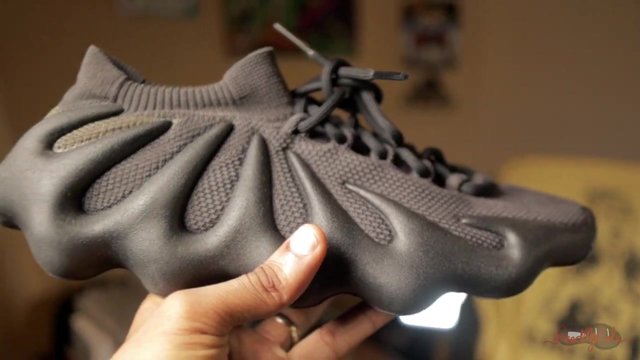 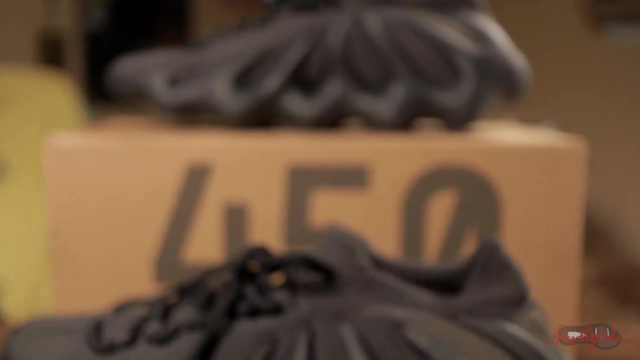 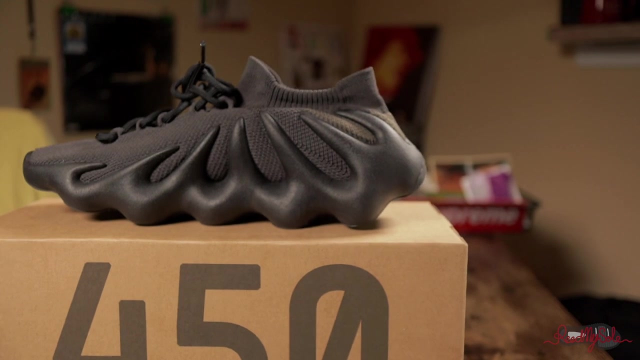 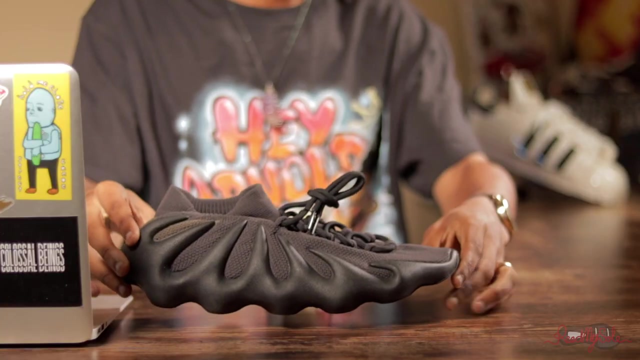 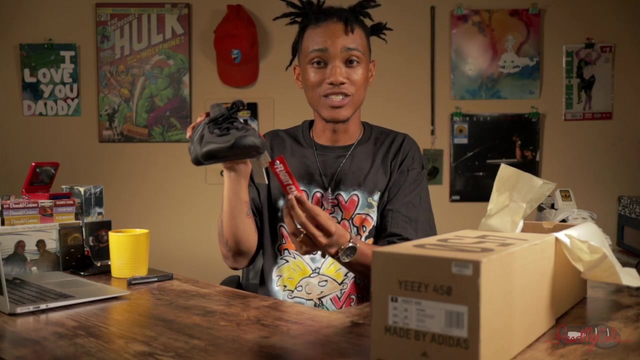 the Yeezy. oh, 450 dark slate right here. you see that? um, you're gonna be that, right there, you're gonna be that right there, you're gonna be that right there. it has the flight club tag on it. as you can see here, it has the flight club tag on it, do not. 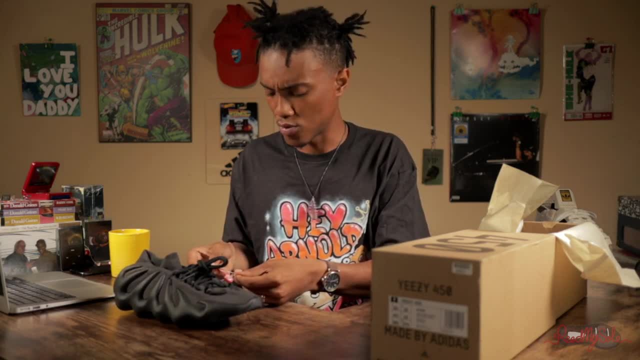 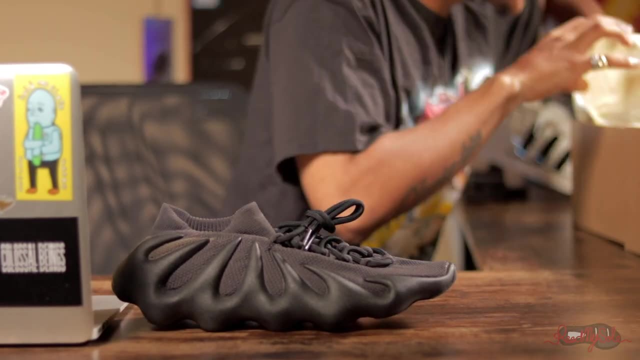 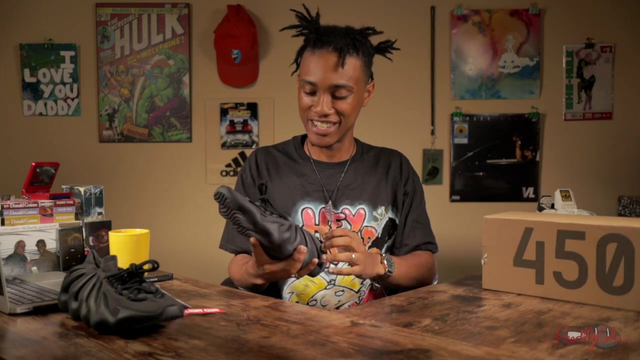 remove tag. this product has been flight club approved. all claims made after this removal will not be honored. we have that right, hey, oh, let's get both of these out. okay, these are very different. these are weird. these are very, very different. babe, you seem like you having an issue. 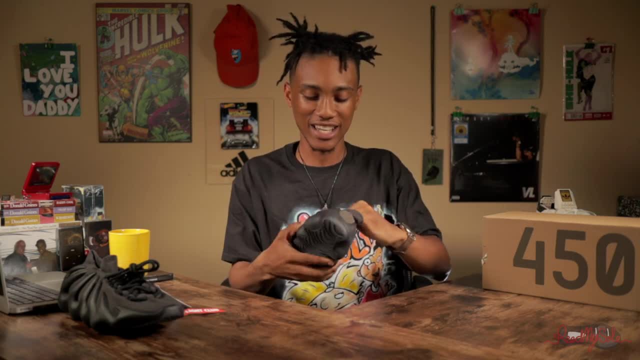 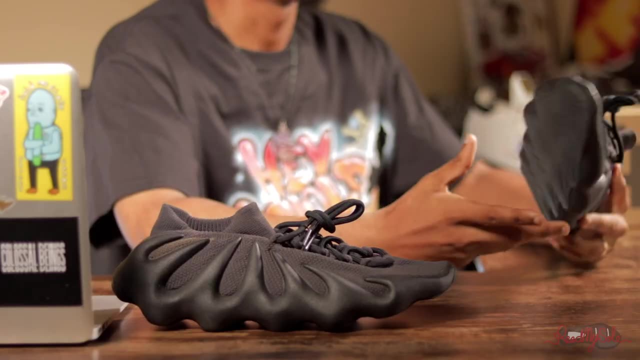 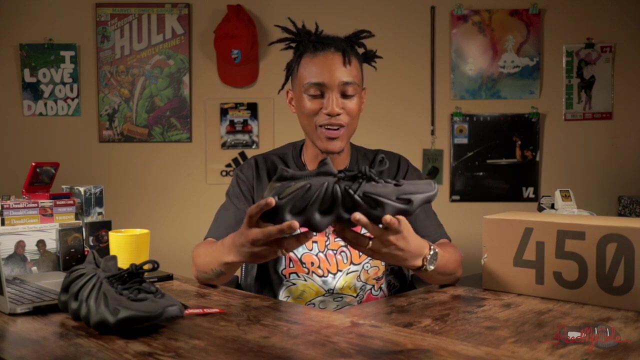 what's going on. my girl is saying they look like cleats to me. okay, to me they're very different. i see why resell isn't crazy for him, but to me it's. it's dope. i don't know what it is about this claw. i don't know what it is about this claw, but it does it for me. it's just something different when. 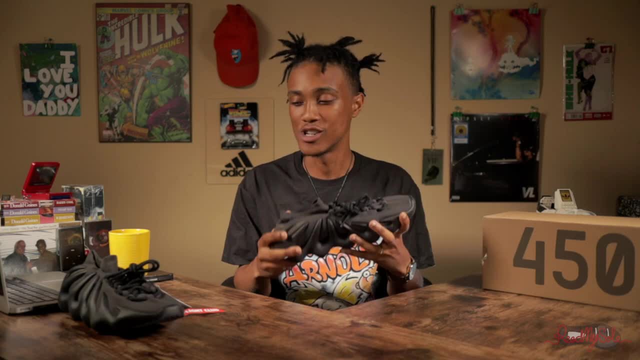 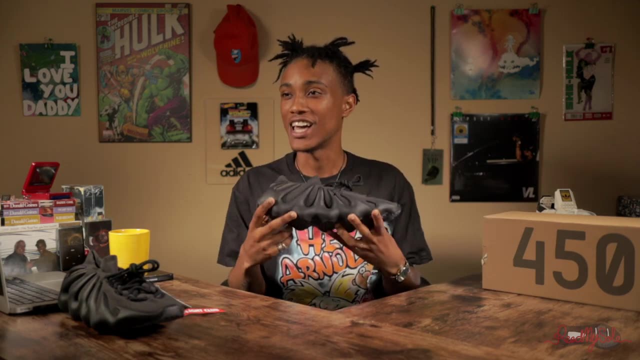 i first saw pictures of this shoe, i really, really, really, really wanted it, especially when kanye west puts it on his feet. i don't know what it is with that man. like i said, he can put doodles on his feet and it will look good. my baby girl right there, hey baby girl, hey mimi, what do you? 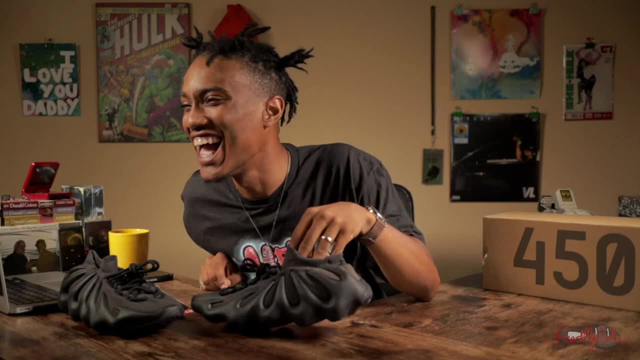 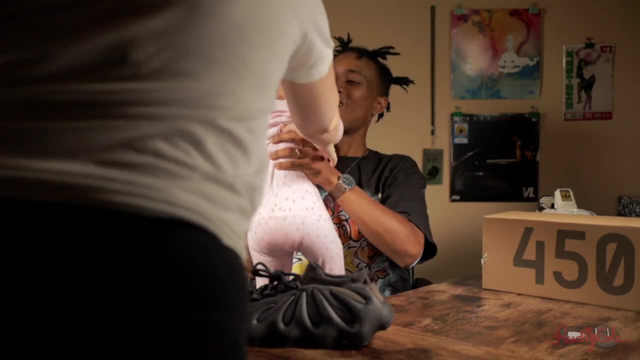 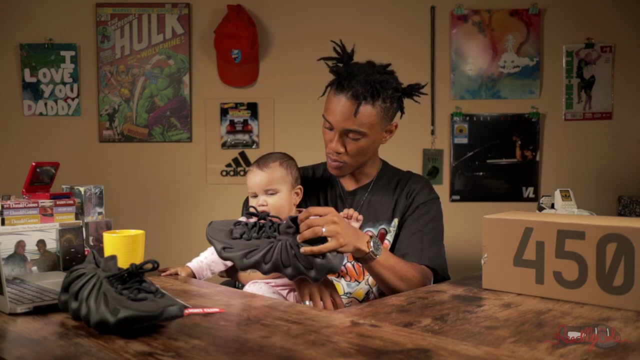 think about these, mimi, how you feel about these? huh, how you feel about these, let me get give me her, make her make a feature. come here, oh oh, say hey, everybody say hey. no, don't touch the heat. what you think about these shoes, mimi? oh, she wants to eat. she's in a teething phase right now. 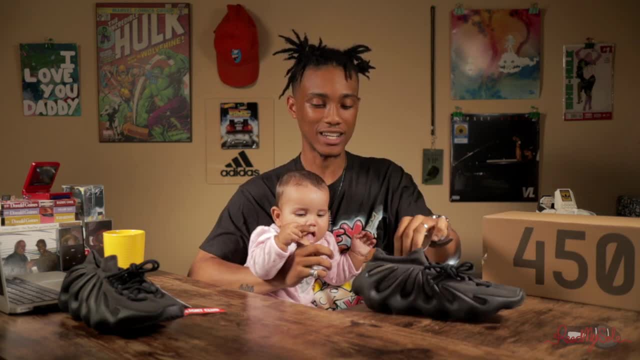 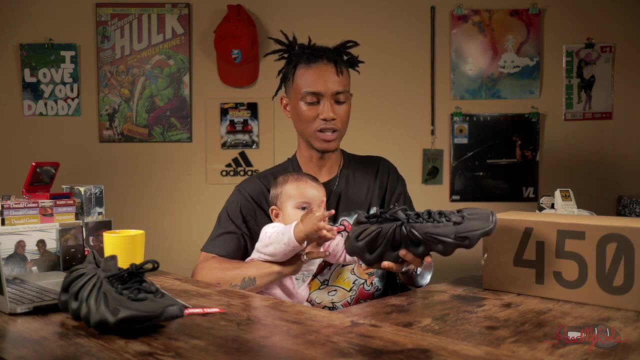 everything to her mouth. yeah, these are the 450. like i said, i got into 10 and a half. you've probably seen full-fledged reviews on them. they're really lightweight but still heavier than i thought they would be. they have like a little bit of like a like a like a chocolate. uh, back. 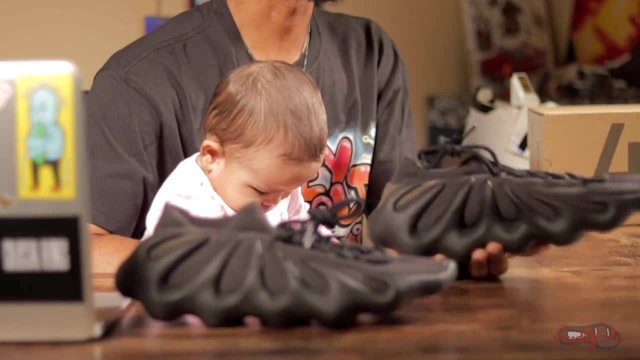 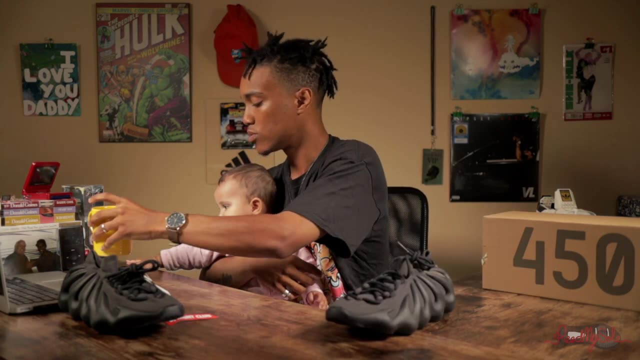 right here. that's like the only thing different other than that is dark, dark, dark, dark, dark and it's like, maybe like a, like an ashy black. i really don't know how to really describe that, but i like them. let's not, let's not spill that baby. let's not spill the hot tea. 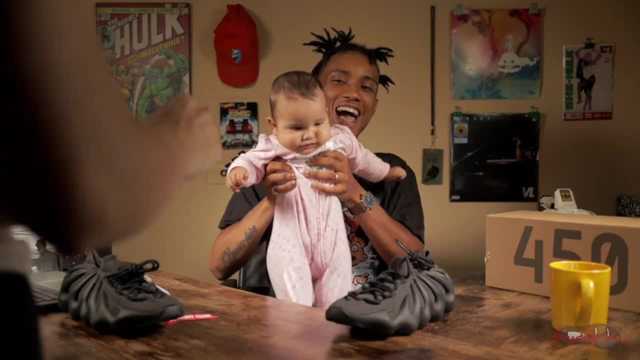 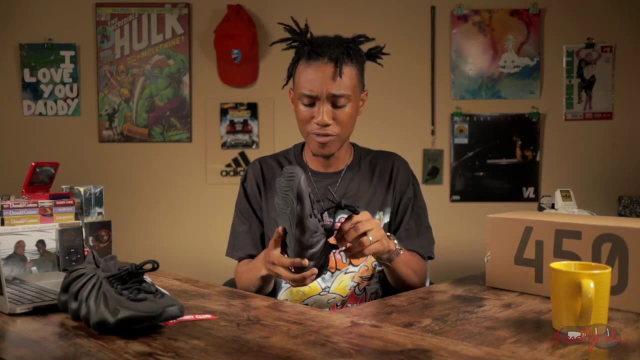 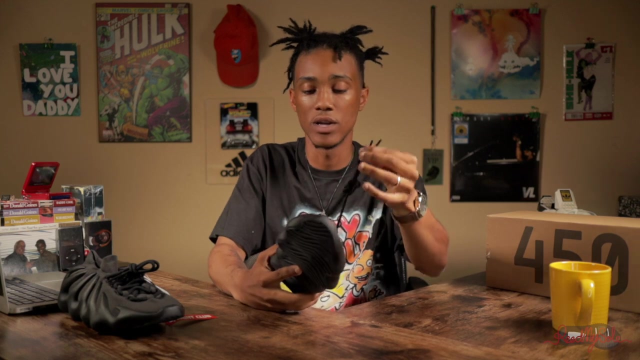 take her back real quick, take the baby girl back. hey, say hi, everybody, come on. so that's mimi right there. yeah, these look very different. these are very, very, very, very different. they look way better on feet than they look in hand. every uh review that i've watched from they look like way different. 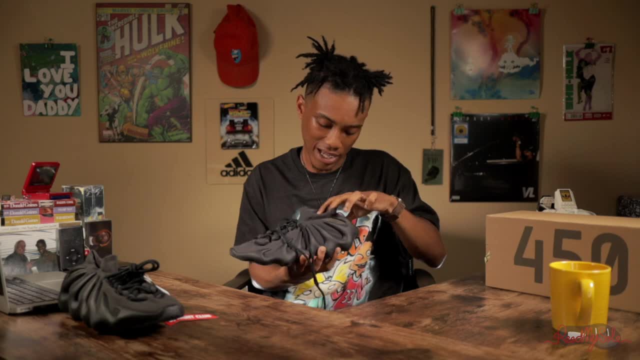 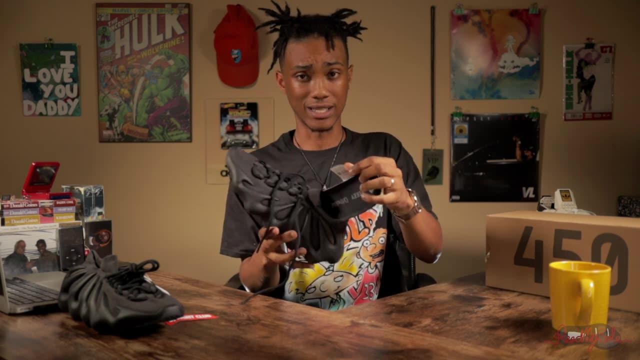 on feet. it has a easy ortholite sole which is kind of hard to like. get in there and see there, you can see, oh. but it has like all of this extra padding and all that good stuff and that's where the tag is at as well. um, it's like art delight and uh, that's where the size tag is at. yeah, man. 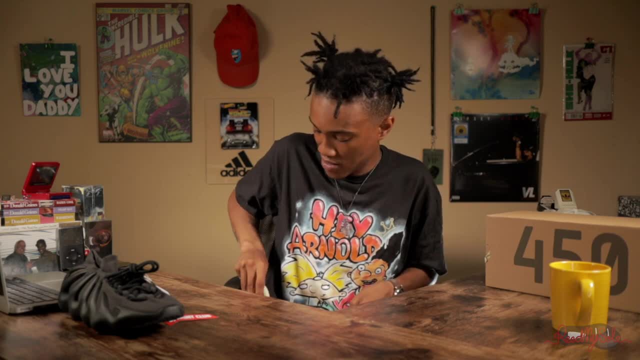 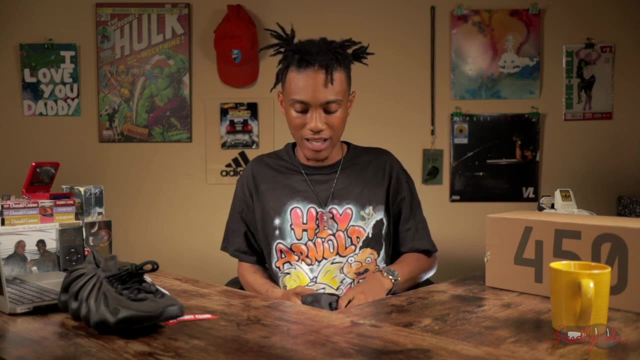 these are, uh, these are nice, i like them. i don't like them in hand right now, but i know, once i put them on feet and i style them with something, that they're gonna look really good. my wife said they look like football cleats- what you say football cleats or soccer cleats, just cleats in general. 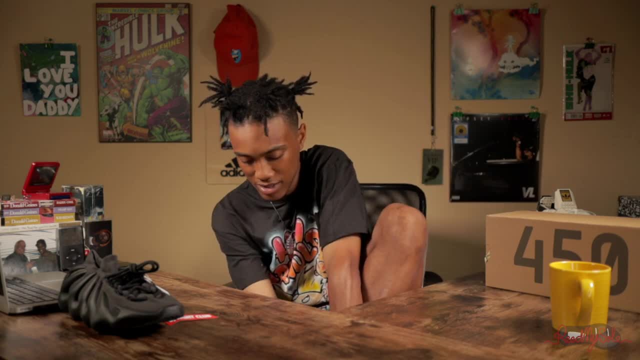 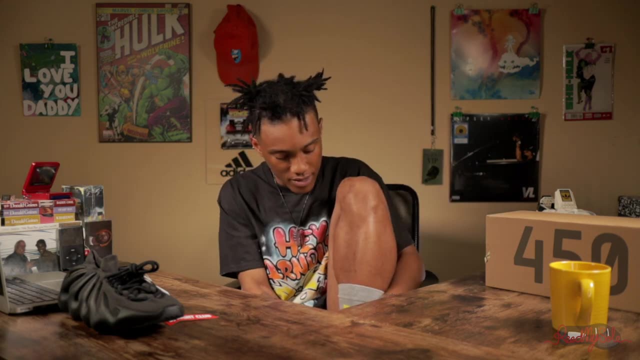 yeah, they like, yeah, they like some track cleats. but let's see these look like, let's see what these feel like on feet. oh yeah, i'm glad i did that. i'm glad i did that. i'm glad i did that. i'm glad i definitely did that. that, that 10 and a half. let me get this on. they'll be straight to the foot. 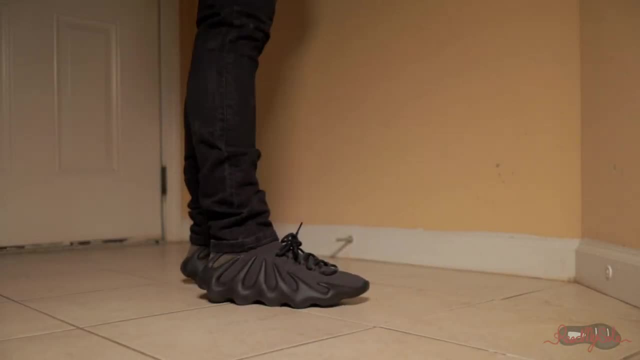 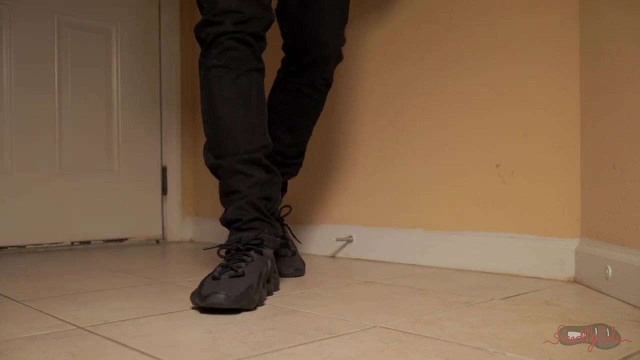 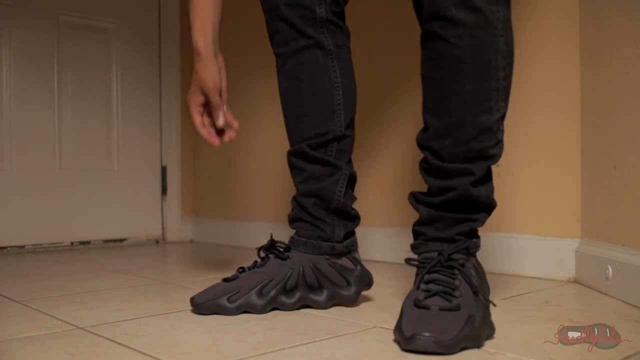 game. you already know how that is. and yeah, the- what do they call this? the medial side looks so good on feet like oh my god, like. i don't know if you can see that, babe, but look at them on my feet now, here, the instep looks so good like, oh my goodness, the outstep looks so good too, they. 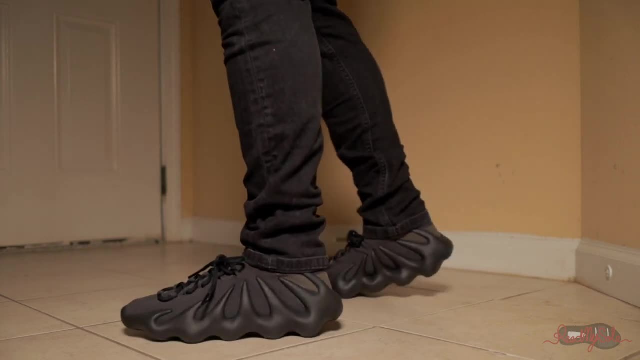 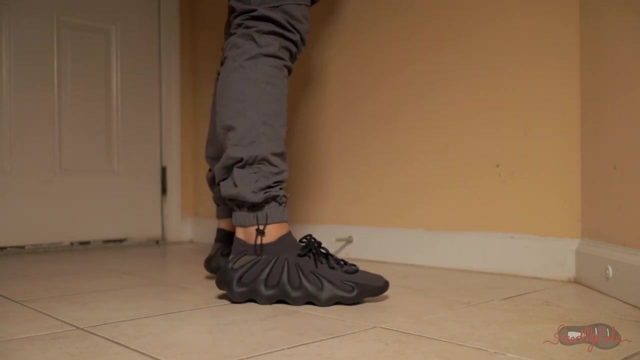 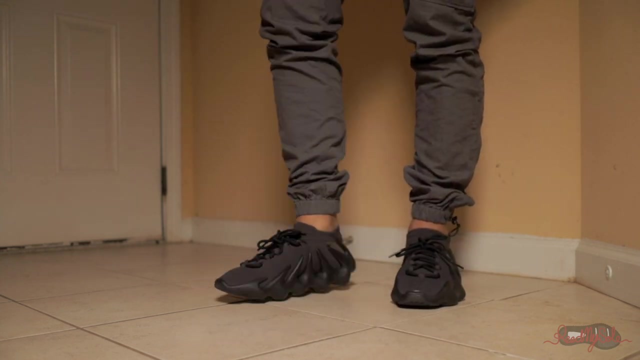 look really good on feet. they look really good on feet. they're a little pointy at the top, but i like them. wifey is not really feeling them, i think because i spent resale value on them. the ankle: yeah, it looks very sock like, but i like it. to me. i knew what i was getting into when i 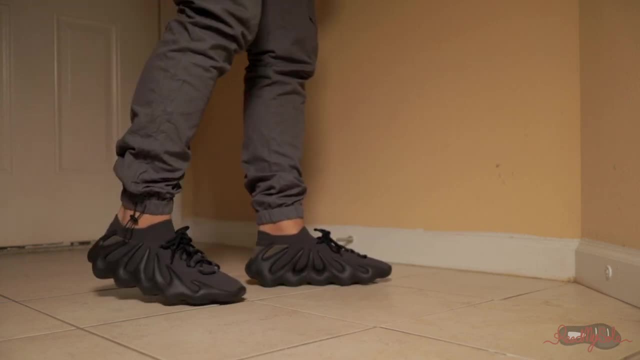 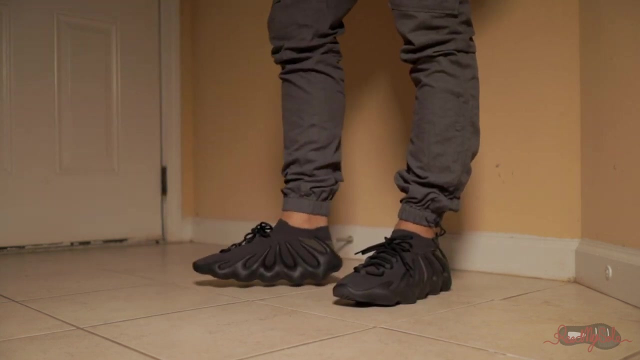 purchased these shoes i knew it was going to be something different. i knew it was going to take some time. but watch, when i style them and i put them on and do the on feet. wifey will feel she will, i i know she will. i know everybody else will. i know what these look like on feet and that's. 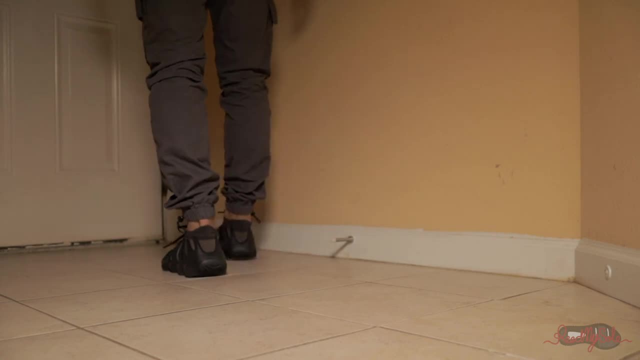 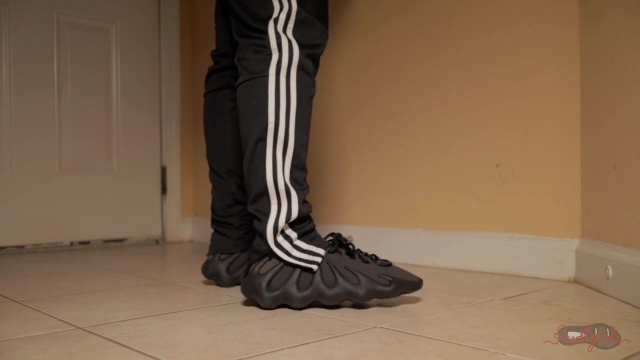 what does it for me? and really it's a different model, it's a different silhouette. i feel as though this is something that is not for everybody and for me it was for me, like i, i really like this shoe. like i said, it looks pretty cool to me. the inside right here looks really cool. it just i. 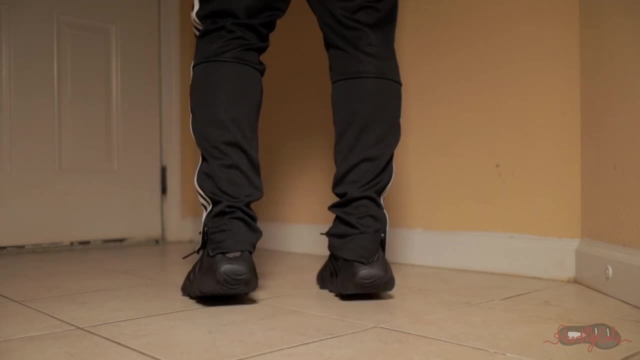 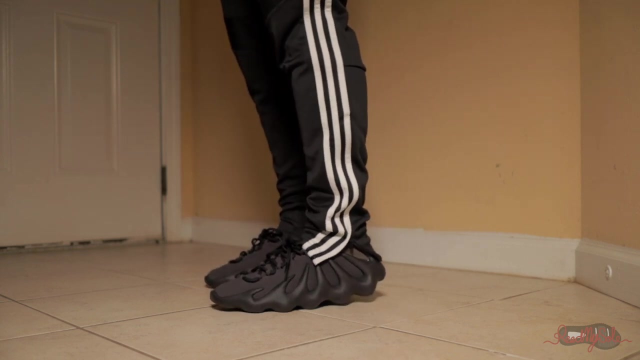 don't know. i don't really know how to describe it. i definitely could have did the 10. i'm gonna say that right now. i definitely could have did the 10 for my comfort. it's. it's, it's good like i have a wide left foot. that's why i put it on the left foot first and i 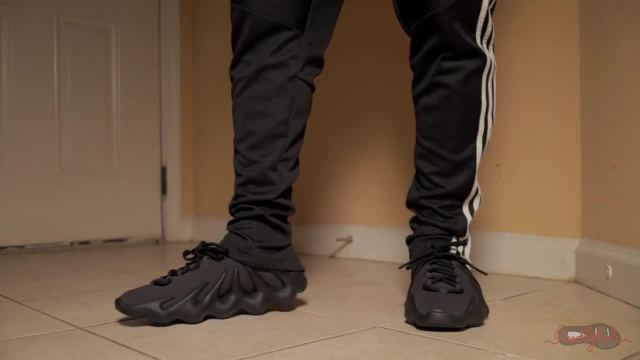 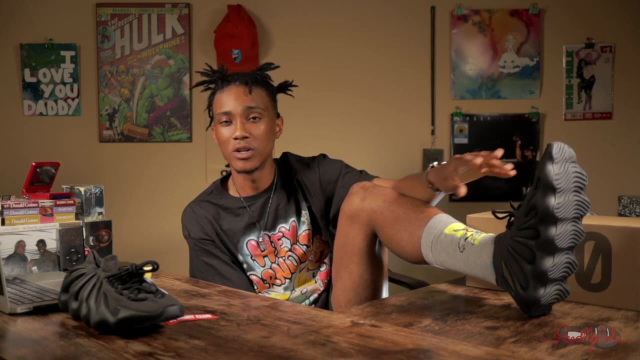 kind of did the 10.. maybe not done the 10 comfortably, but there's still some space, like there's still a little space right there. so i definitely could have did a 10. probably it probably wouldn't have been comfortable, but i would have been able to do it. maybe not wore them. 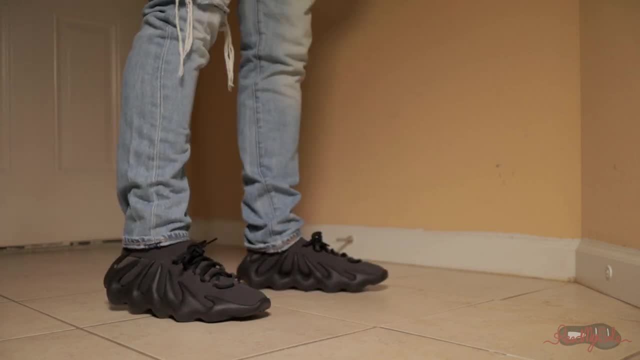 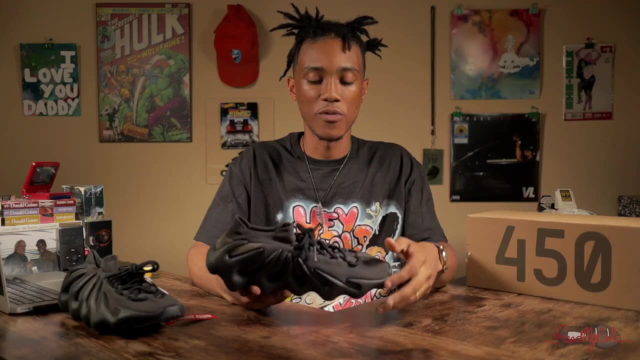 as much or as long, but i really like this shoe. man. this is um something different. like i said, it's not for everybody, but, um, i think, over time, when i wear them or when i you know, i don't think it's a good short shoe. i don't know why people 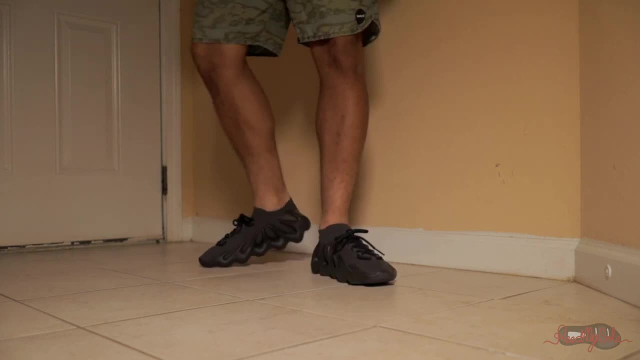 wear these with shorts, but to each his own. to me, this is a good shoe. it would have been really dope to have it, maybe a high top or something else, i don't know. i like it, i think it's cool, but i think you should cover this. i think you should definitely cover this with some pants. um, this is definitely. 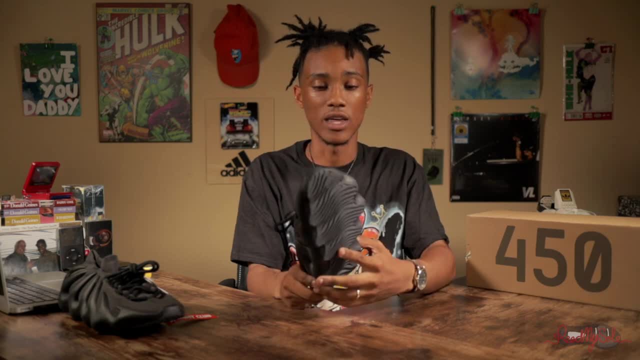 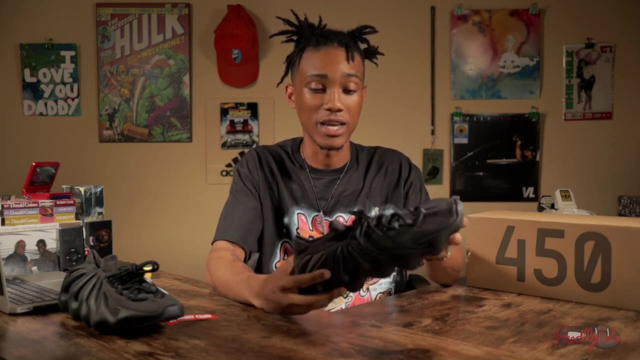 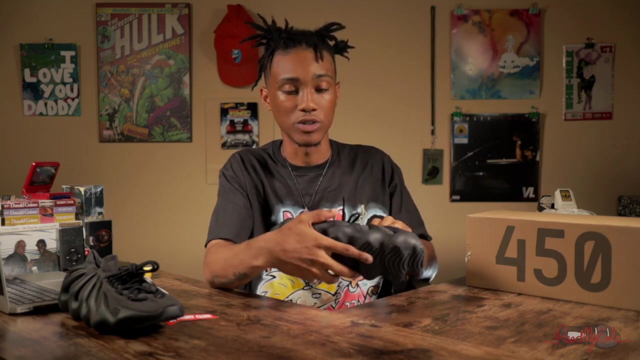 going to be something i'm going to kick around in the wintertime. this is something that i really wanted because it's so different, because it's uh, it's made in germany. it's made with algae. this is like um, algae right here. this soul is like really, uh, biodegradable. so that's something dope for me, and i think it just looks. 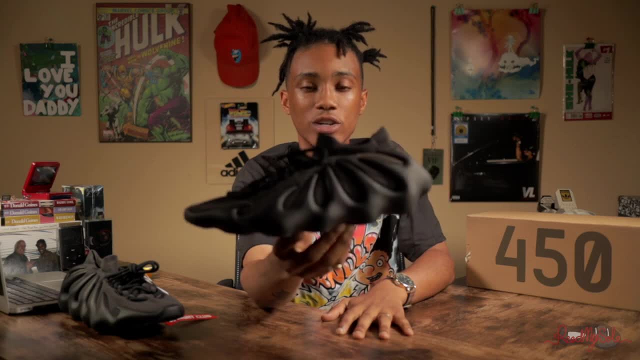 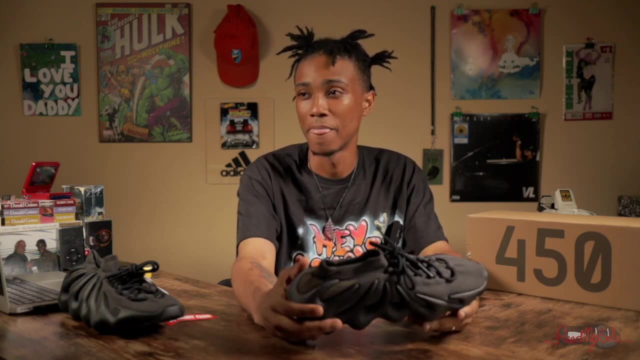 good, i don't know, i don't know it. it may look weird to you, it may not look the best to you, but to me it's something that i like. i'm a pants type of person. like i don't really like wearing shorts, i don't really have many shorts. i like wearing pants. for me, this is something. 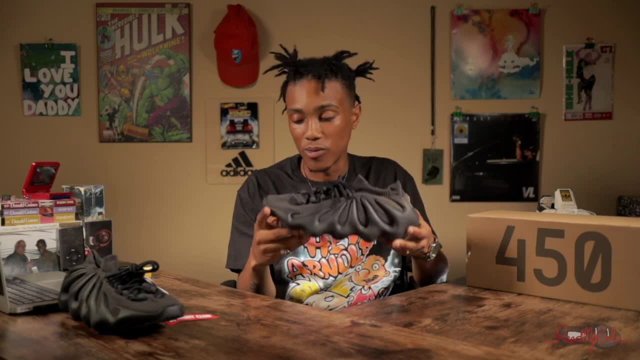 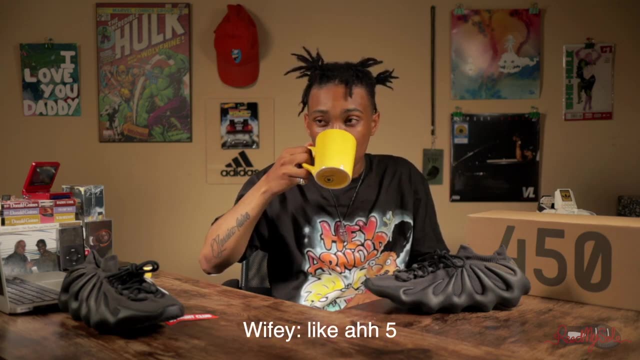 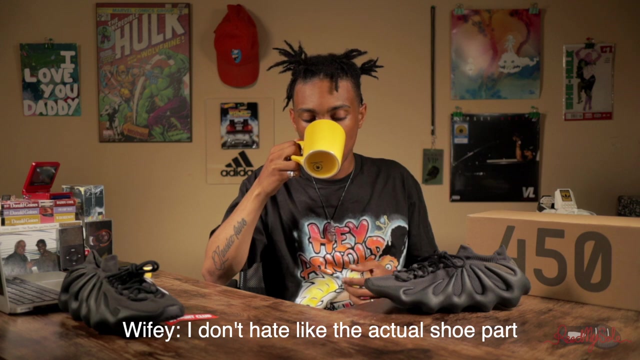 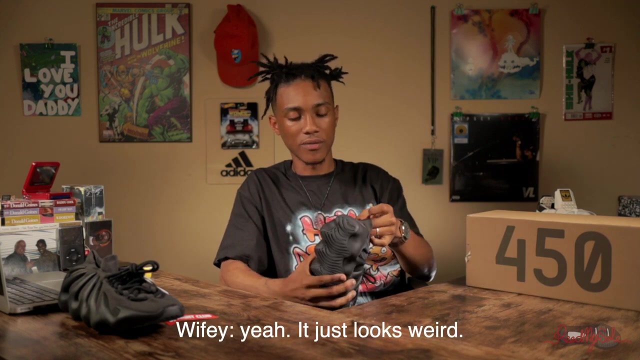 i'm looking forward to wearing in pants, wife, what, what, what are you giving these? give it an honest. be honest right now. like, uh, like a five. like a five, okay, that's not terrible, i don't hate like the actual shoe print. i just want like the ankle part, the ankle, the sock, yeah, okay. 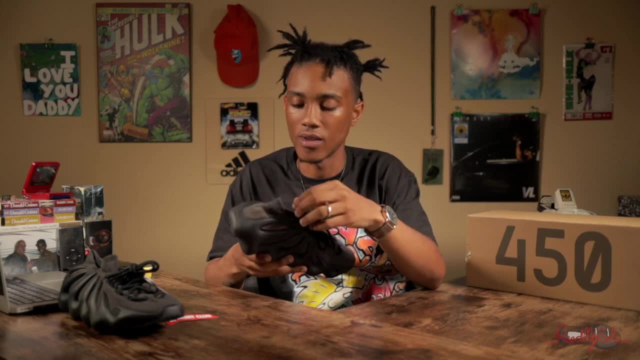 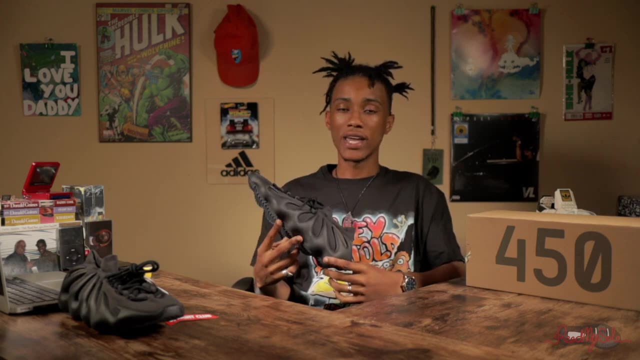 well, i don't know if you're supposed to wear socks with them or not. definitely you're not supposed to show the socks to me. i don't know if you're supposed to wear socks with them or not. me personally, i think these look way better on women's feet- smaller women's feet in a way i wish. 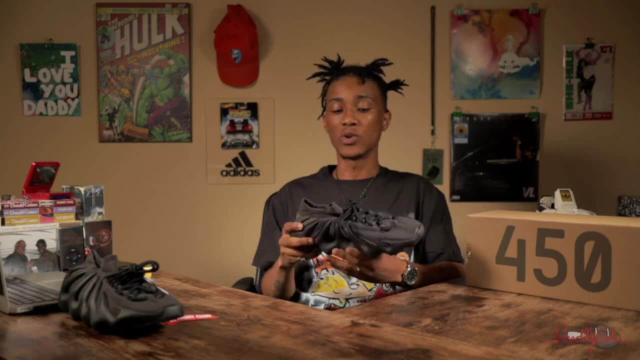 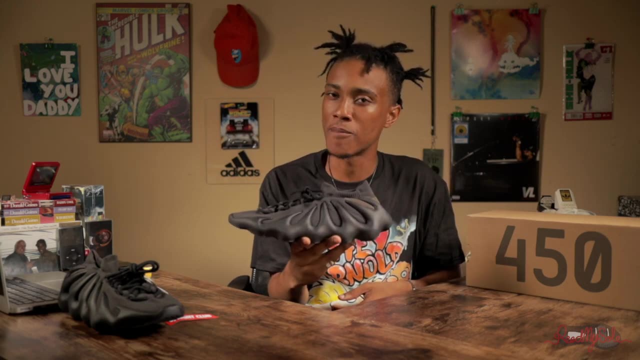 i would have went with the 10 and then, in a way, i'm glad i didn't because i want to wear these. this is my first all black. easy like this is my first. one of my first all black shoes. i don't want to talk about the last time. i didn't get the all black shoes. my brother talking to you. 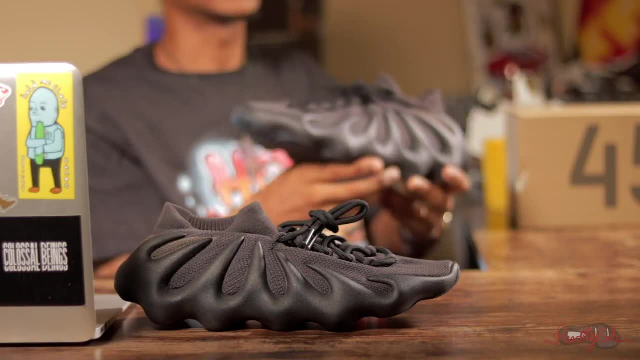 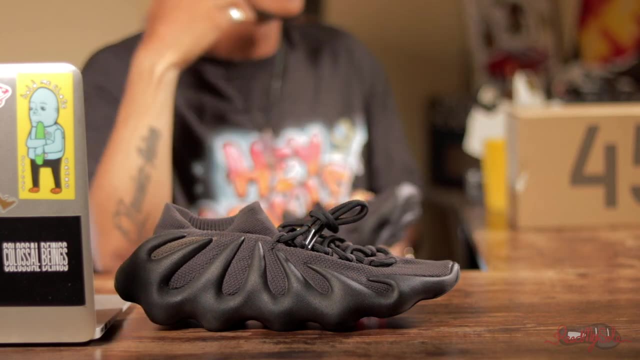 dashawn, i don't want to talk about that. i really want a pair that i can just wear without thinking right, still be, fly, still be dope, and just toss on and don't have to think about them getting dirty. i have a thing for lighter shoes. those are usually my favorite go-to shoes, which they really get dirty because i wear my kicks. 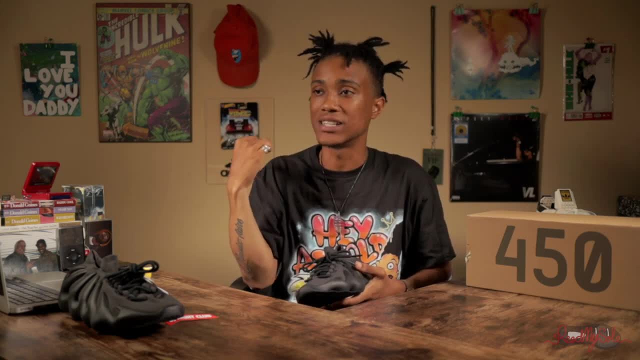 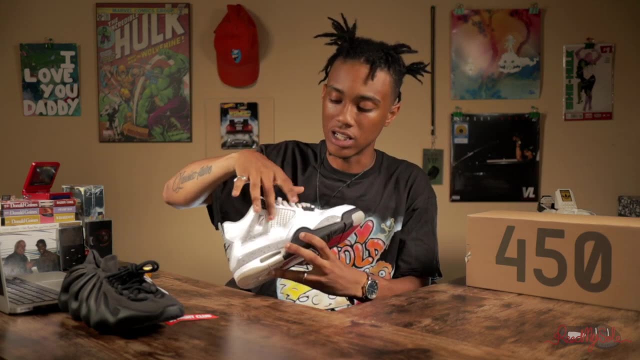 so even like my white cement fours- i haven't wore those as much, but i've worn them. you get, i'm saying i'm wearing them over the time and over time, even if you don't wear them crazy, they still start the yellow and they still start to get off colored and stuff like that. and even though this 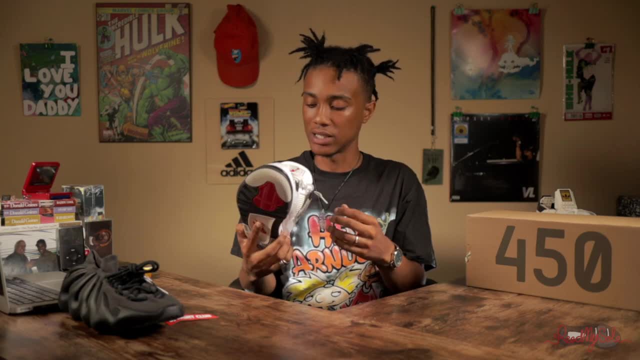 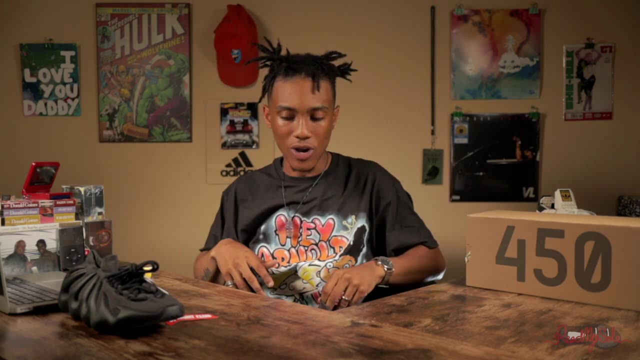 still looks good and to me it's not the best looking shoe. i mean i still got the nike air in in on the insole. so you know i wear them, but i try not to wear them too much because white shoes get crazy. so for me this is something that. 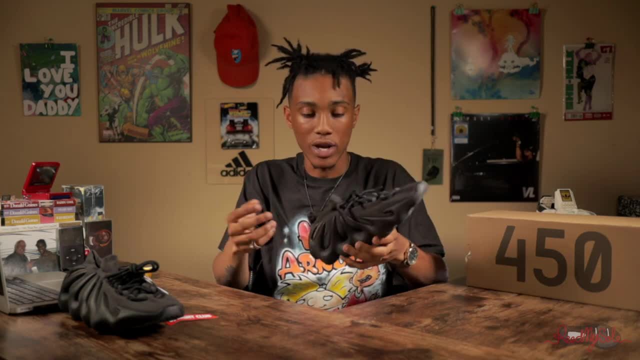 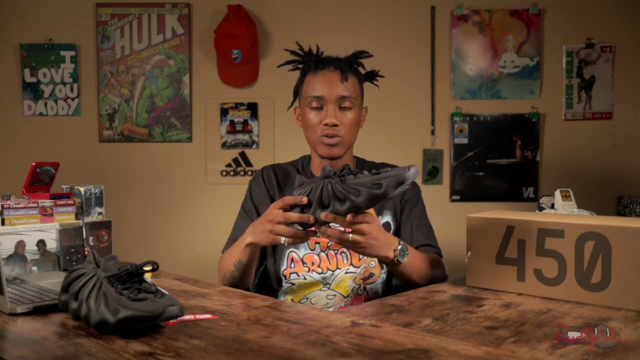 i'm looking to just throw on. we're going to a wedding in a in a few a month, and this is something i just want to wear and, you know, just wear around and kick around while we go do things, while we go do activities, you know, while we go to the zoo or while we go to the park or something like that, and 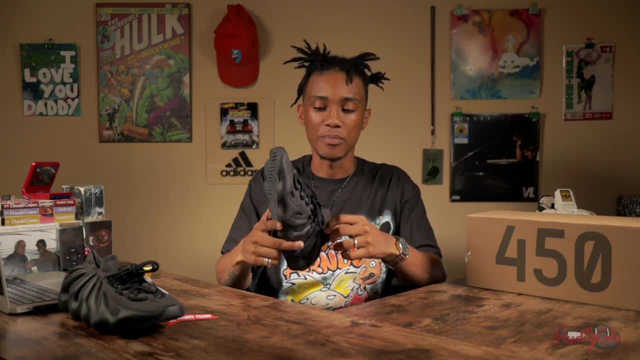 i know they're not going to get super dirty and they're going to look really clean- and people are. i'm still going to break them next and be like: what are those? because these seem like a. what are those shoes? tell me what you think about them and i'll see you in the next one. bye, bye. 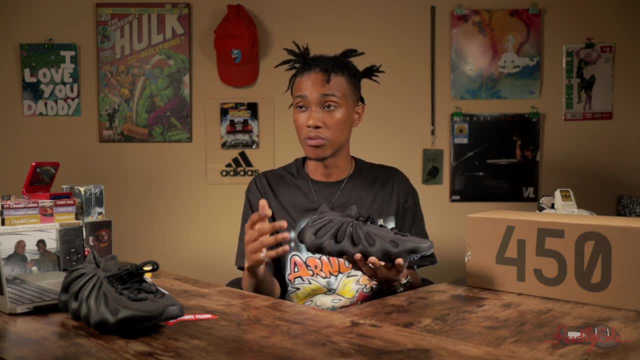 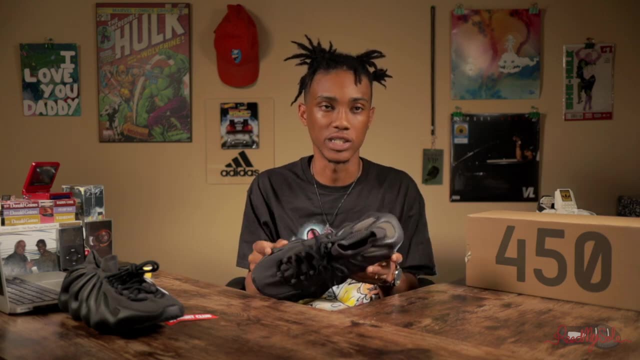 think about on the on feet section. i think that the on feet section is going to make or break this for some people and i am going to look into getting actually after this, i'm probably going to look into getting something from h&m or look at what i have in my closet right now to kind of 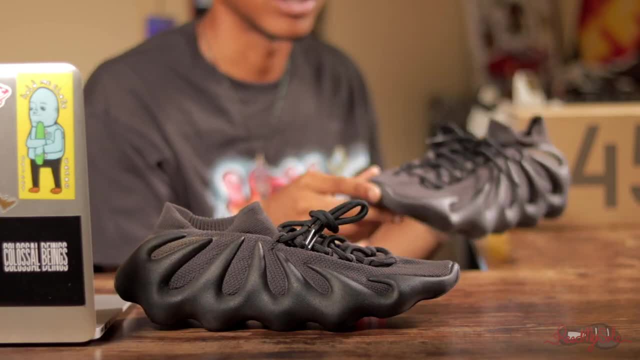 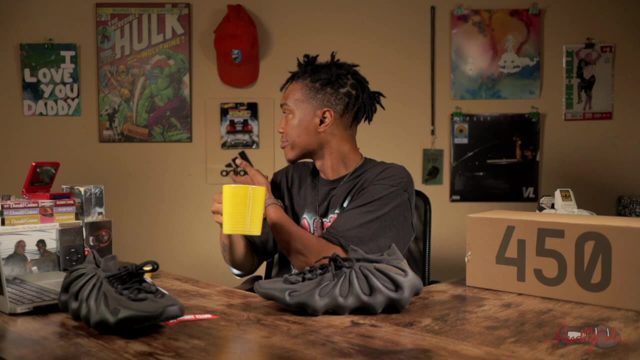 make these look good and get to sell you people on it, because you know i obviously work for yeezy brand now without getting paid. adidas, the adidas superstar lego, like it's crazy. make sure you comment, like, subscribe and i'll see you in the next one. bye, bye. 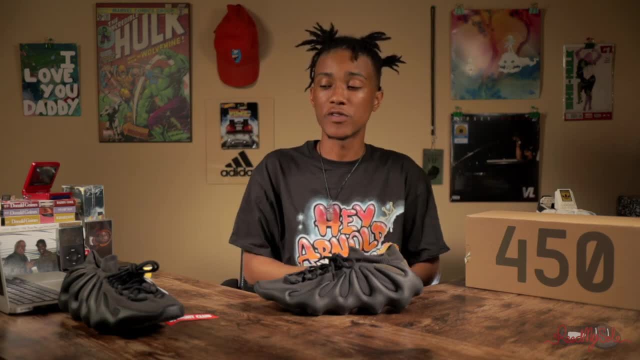 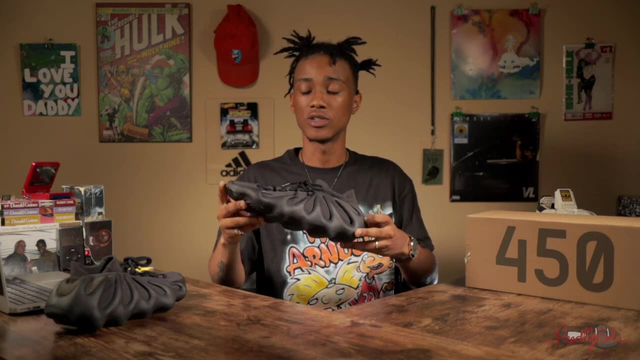 subscribe. tell me what you think about these shoes in the comments. like i know, they're not for everybody, i would suggest um for sizing, that depending on how you feel you can go true to your size. i could have definitely went to a size 10 and been okay. it probably wouldn't have been the 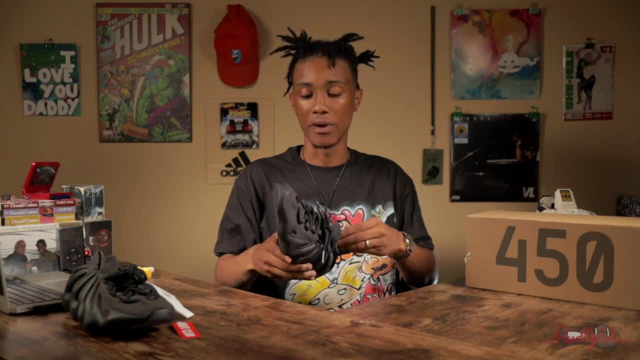 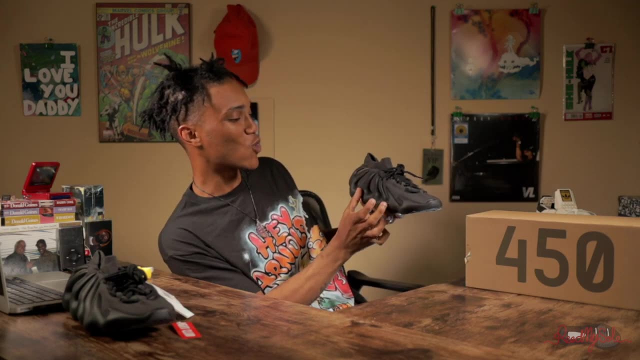 best. probably wouldn't have been the best feel for all day wear, but i could have did that and been fine. this side is just so fucking sexy to me, like that instep is just so to me, um, but yeah, i think these are re-releasing anyway by the end of the year. uh, i'm not sure if i'm going to be able to. 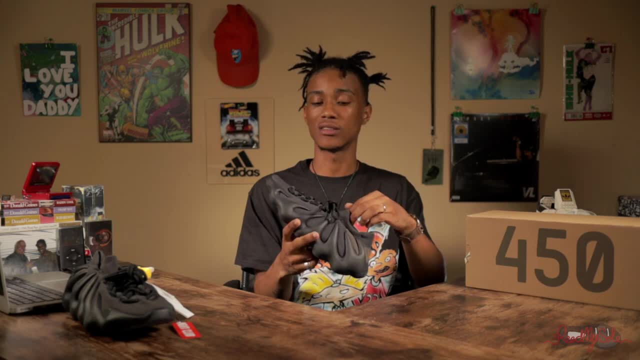 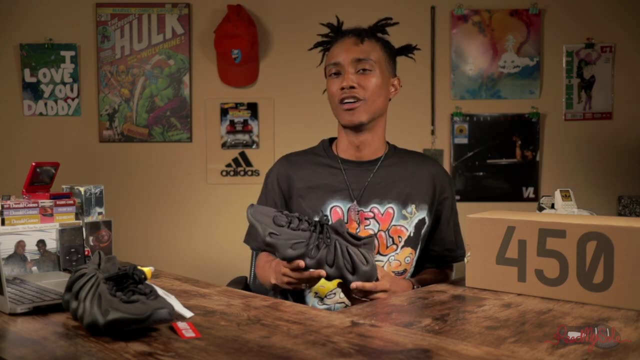 what i heard is that they're going to re-release. but if you just like anybody else, these are really popular. these 450s are really popular. you know, when kanya comes out with a shoe, everybody's like oh, but then they always sell out. so it's just like: why can't i get them for retail? yeah, this is my.